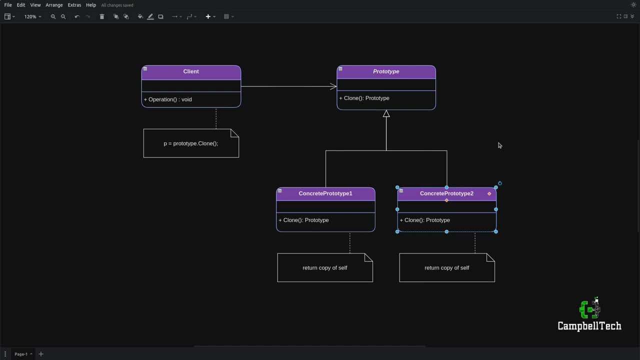 minor modifications, then you can simply go ahead and clone or copy that object and then make the desired adjustments, and this will be a much faster and convenient process. Now let's go ahead and look at our particular use case, and then it will make more sense. 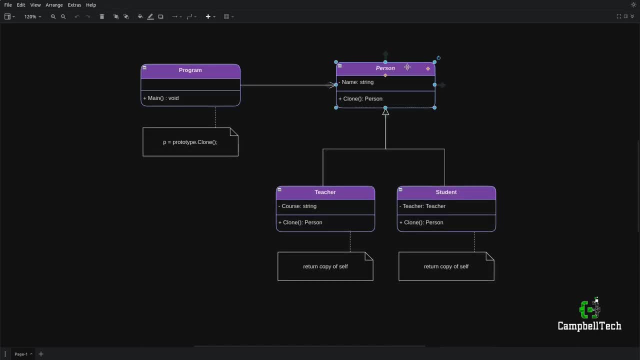 Now our use case will be based on a person. that can either be a teacher that teaches a given course, or it can be a student that has a particular teacher that teaches a particular course. but more specifically, when we focus in on the prototype design pattern, the person class is an abstract class. 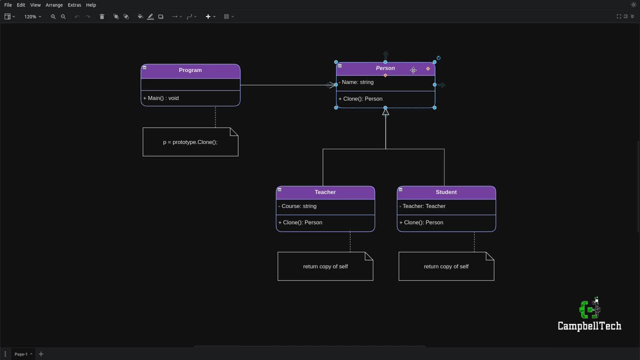 that takes on the role of the abstract prototype. now you might say i said that the abstract prototype was an interface, but it can be either an interface or an abstract class. and then it defines the clone method that allows the client code to clone a teacher or a student object, and then the 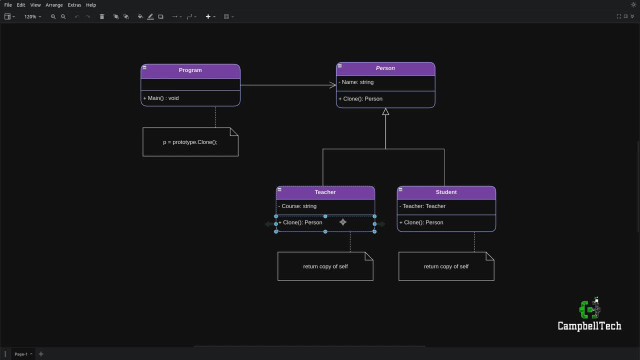 teacher implements the clone method, and when it is invoked, it will return a copy of itself, and the student or the teacher will then use the clone method to clone. the teacher or the student object also implements the clone method, and when it is invoked, it'll return a copy of itself too. now you 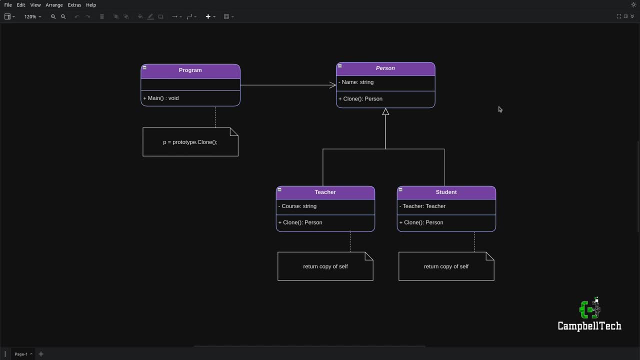 might say that you said it's useful when you construct an object that takes a very long time to build or when it is very resource intensive to construct an object now. first of all, it goes without saying that a person like you and i is quite complex. so if we had to create an object, 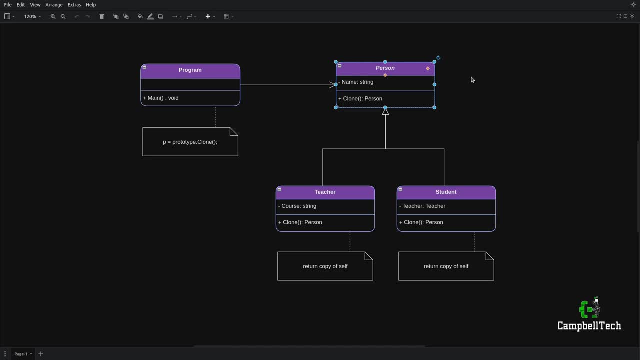 that contains all the attributes of a real human being. it would be entirely complex, but, as mentioned before, i like to use very simple examples so that the focus is on the design pattern itself, in this case the prototype design pattern, and not on some fancy implementation that might distract. 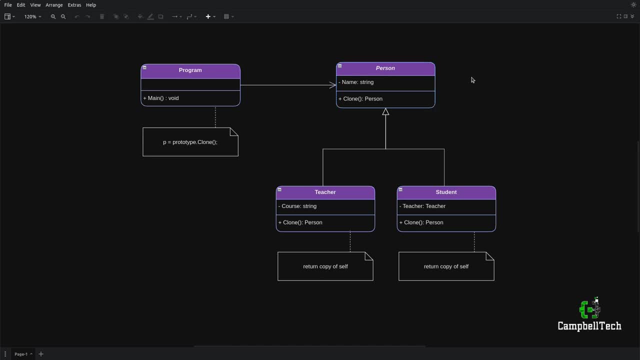 you from completely understanding how the pattern works. so now you've seen the class diagram next up, we are going to write the code, and if it hasn't made sense from the class diagram perspective, i'm certain it's going to make sense when you actually code the prototype pattern. it is now time to code the prototype. 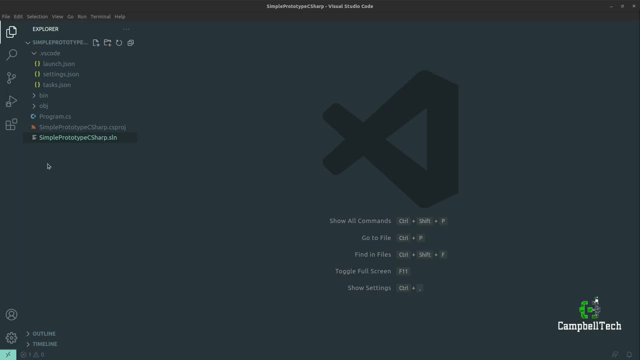 pattern. the first thing that we need to do is to create our prototype or abstract prototype. so let's create a new class and call it person, go ahead and make it an abstract class and then let's mark it as the prototype. now, as you can recall from the class diagram, we need to define a clone method and that clone 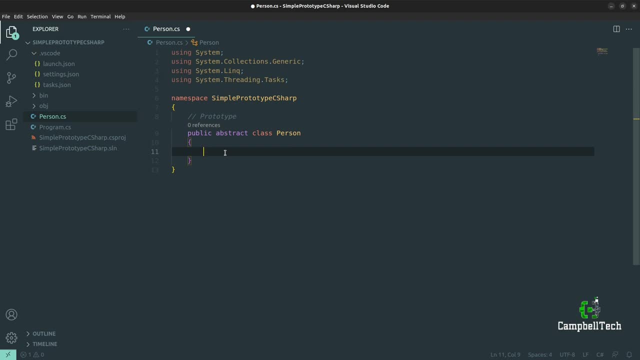 method needs to be implemented by the concrete prototypes and since we are using an abstract class, we are going to make it an abstract method that forces the subclasses or concrete classes to implement this method. so let's say public abstract. it needs to return the same type as the prototype and that's person, and let's call it clone. 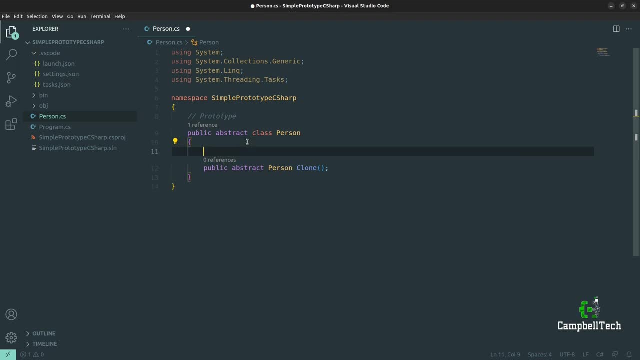 okay, and then i'm also going to add a property for a name, because a person has a name, whether it's a teacher or a student in our case, and that's also the reason i selected the abstract class rather than the interface, so that we could share the name between the teacher and student. 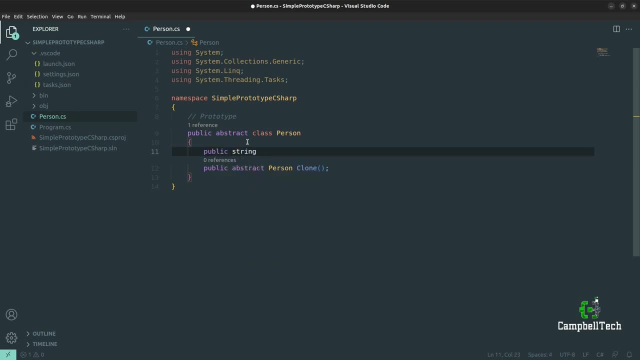 objects. so let's say public string name, and then i'm going to use the auto property syntax there i'm also going to create a protected constructor. now, the protected constructor will only be accessible via the subclasses. let's pass in a string parameter and then let's simply 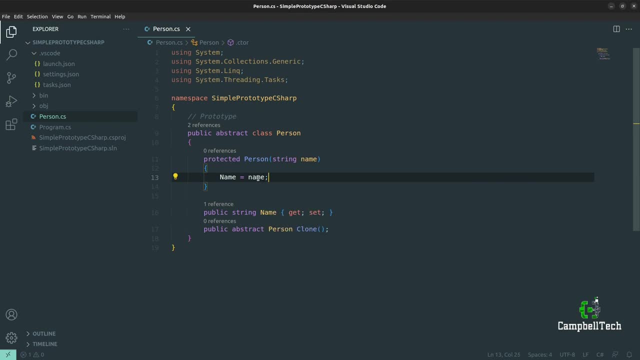 set our property okay, and that's all we have to do in our prototype class. next up, let's create our concrete prototype one. so let's call it teacher, let's extend the person class and, before we implement the abstract method, let's mark it as our concrete prototype one. 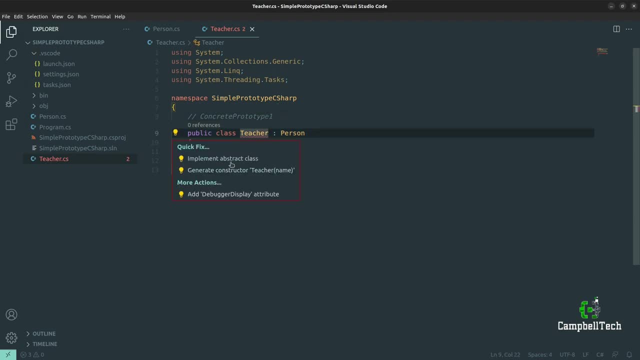 next we can go ahead and implement the abstract class, in other words the clone method, and then you'll see that it also expects us to pass the name parameter to the person classes constructor. so before i do that, i just want to add another property to the teacher. so a teacher will teach. 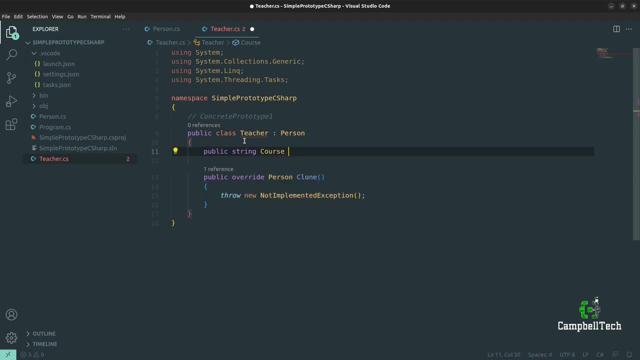 a course, so let's add a string property for the course name, okay. and then let's go and add a public constructor for our teacher, so say public teacher, and then it's going to take in the the name, that will pass to the base and it will also take in the name of the course. 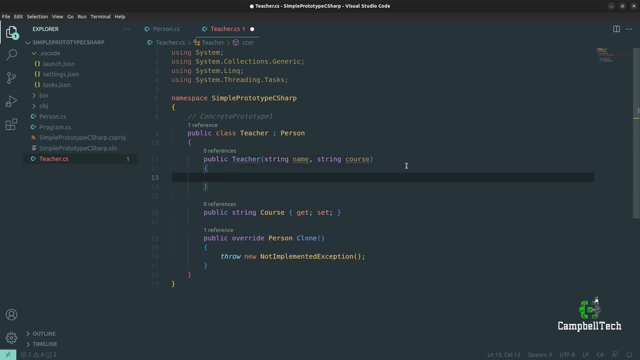 okay, the name will pass to the base, like i said, and then we'll set our course property here. okay, so now we have our teacher object that contains a name that it gets from the person base class and a teacher also teaches a course. so for us to clone this we can conveniently use. 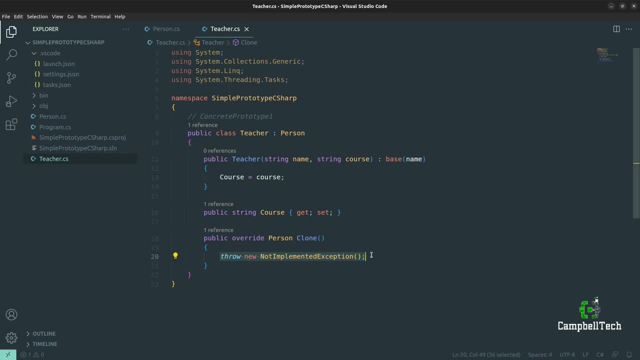 the member wise clone method, that is, on the object class. now most of you will know that each and every class in dot net, for example, this teacher class extends object or in this case, the person class extends object and the teacher class extends person that extends object. so you'll see what i mean just now. so let's say return. 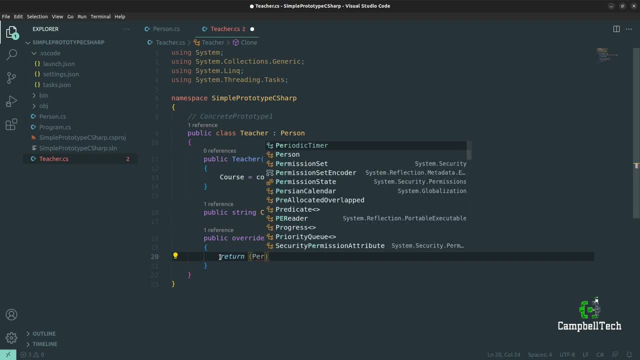 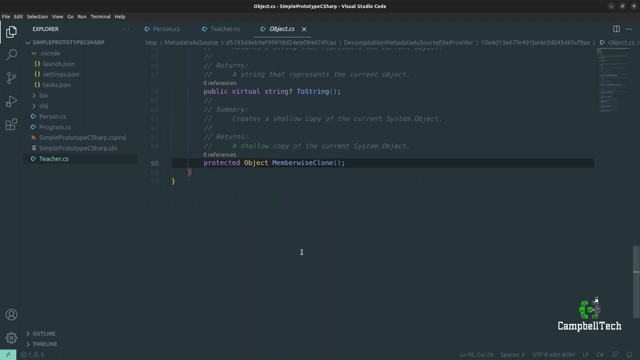 we are going to cast the memberwise clone to the person class, our prototype, and let's say member wise clone. that's a method on the object class, like i mentioned. so let's go to the definition and here you'll see that the memberwise clone method. 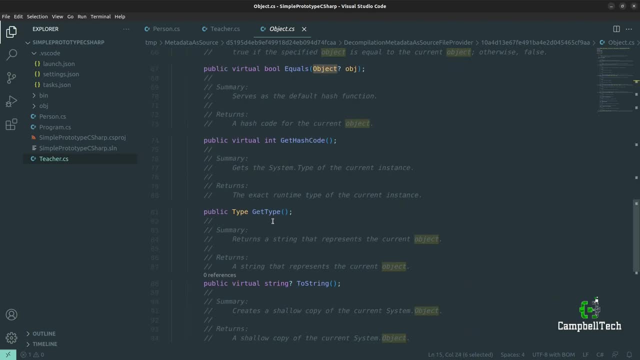 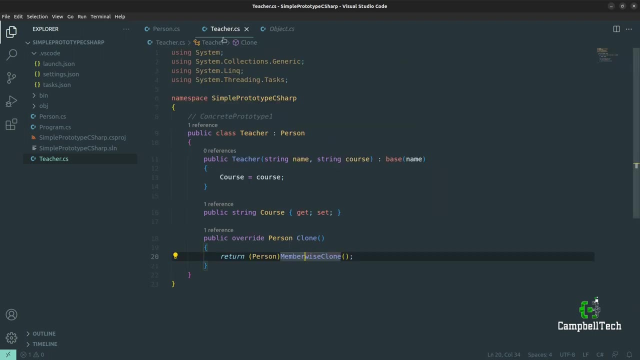 is in fact, on our object class and its purpose is to create a shallow copy of the current systemobject, but in this case it'll be a shallow copy of the teacher class or specific instance of this class. okay, so this is all we have to do for the teacher. 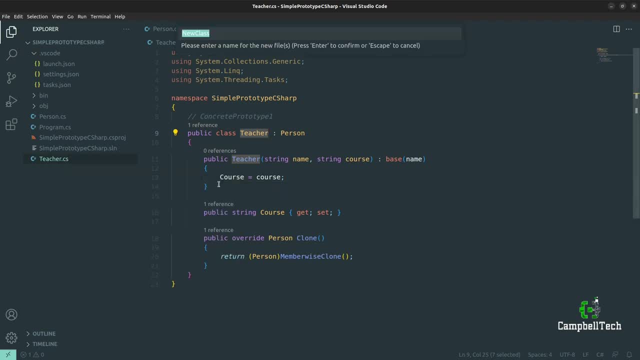 class, our concrete prototype one. so let's create our concrete prototype two, and that is our student class. again, go ahead and extend the person class, our prototype, and then let's mark this as our concrete prototype two. implement the abstract class. okay, again, before we implement our clone, 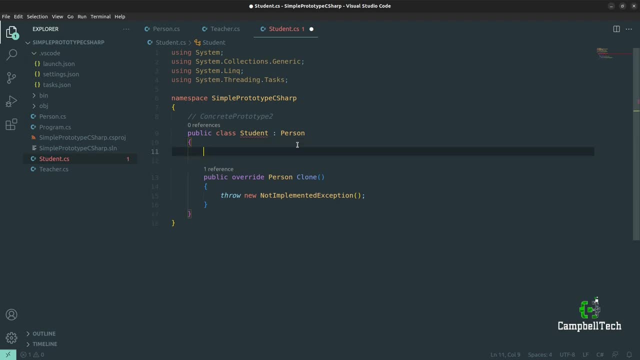 method. let's just define our student object. so i want to go ahead and add another property and that would be a teacher. so we can say: public teacher, call it teacher. so we are saying that a student has a teacher that teaches a course, okay, and then we need to generate a constructor. 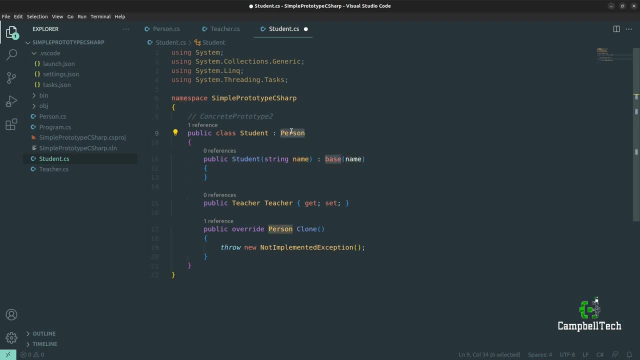 again, we are passing the name to the base, our person class, which is our concrete building class, our prototype, but we also want a teacher parameter to be passed here, and then we'll simply set our teacher property in the constructor here. okay, so this is how our student object will look. 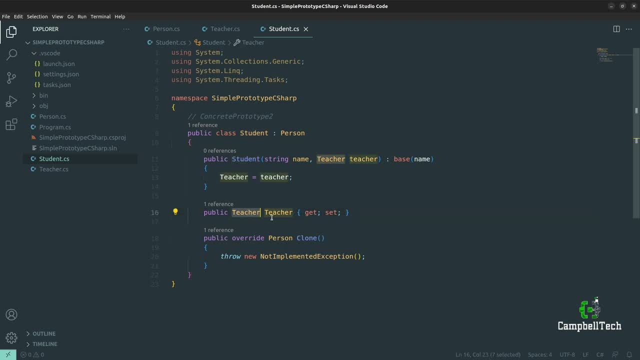 now there's no particular reason why i added the teacher, our concrete prototype, one object, in here, so that's not a rule by default. i just wanted to show you what will happen if we use a reference type or complex object rather than a primitive type, and you'll see what i mean when we test the 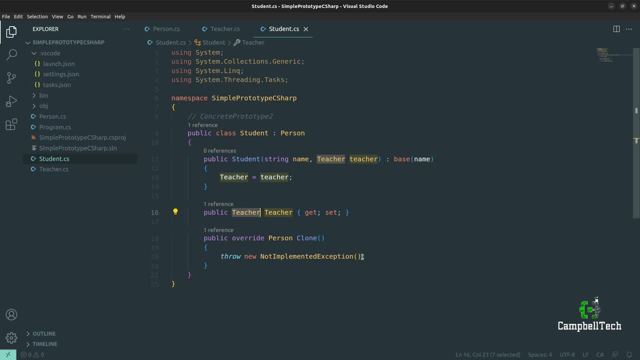 code and it's got something to do, as a hint for now, with the shallow copy, or rather a shortfall of the shallow copy, and you'll see what i mean in a minute. okay, and then let's implement our clone method. we can say return, return, and then we'll say, member wise, clone again and we'll cast it to person. 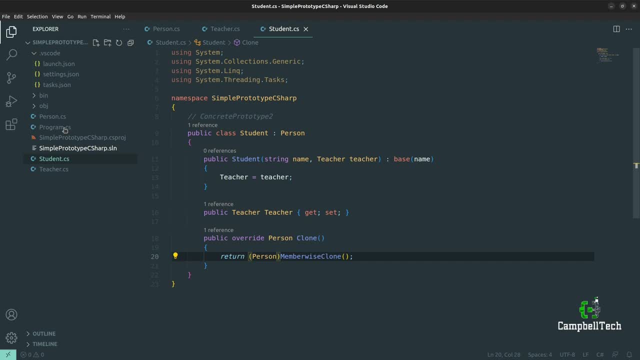 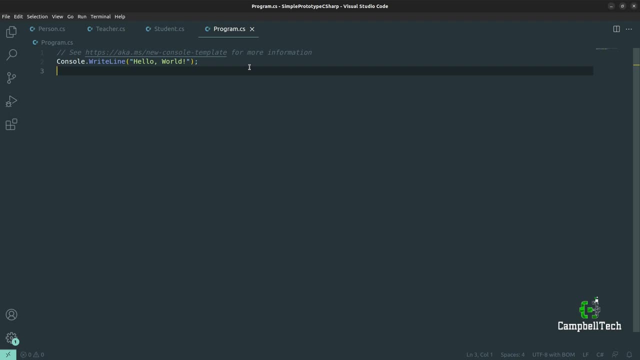 okay, and that's all we have to do, so we can head over to our programcs class. okay, and then the next thing to do is to write our client code here in the programcs class. so let's start by saying: teacher, go ahead and add the user. 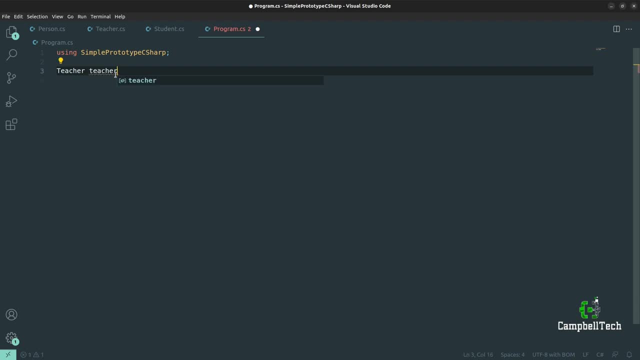 using statement and then we're going to instantiate the teacher object only once, okay. and then let's pass a name. i'm going to pass my own name and then i'm going to say that i am teaching a course, something like creational design patterns in c-sharp. 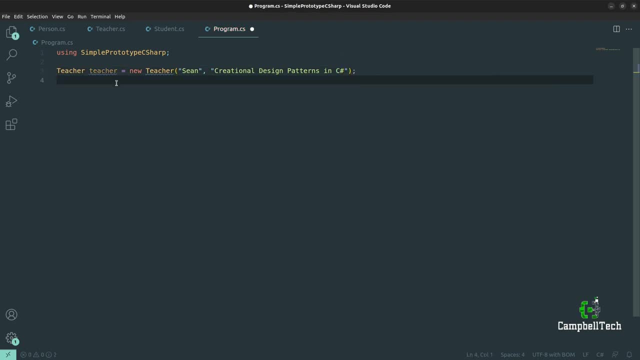 okay, and then we can make a clone of this teacher. now roslyn is telling me that i can use the new expression so that it looks like that, which actually means new teacher, but i just want to use the old syntax and then let's say teacher. now, this time we're going to make a clone, so let's call it teacher. 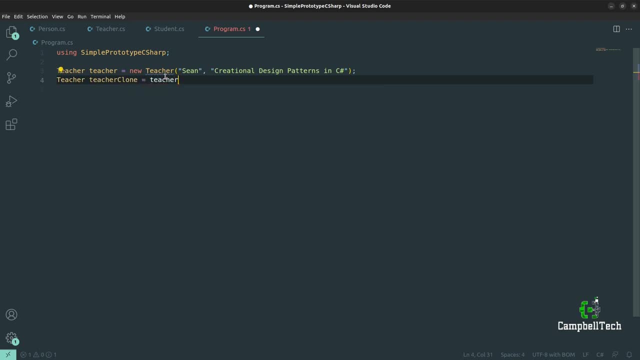 clone equals teacher dot clone. now it returns the abstract prototype person, so let's cast it to teacher. okay, so we have now successfully created a clone by invoking the clone method on the teacher object. and then let's print something out to the console: console dot right line. 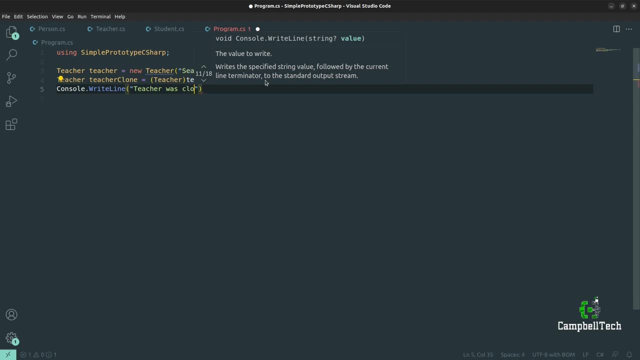 we can say: teacher was cloned, and then i'm going to use string interpolation. then we'll say: teacher, clone dot name, who teaches t a clone dot course. okay, then we can go ahead and do the same for the student object. so let's say student. this is our concrete prototype. 2 equals new student. we'll say: our student is called james. 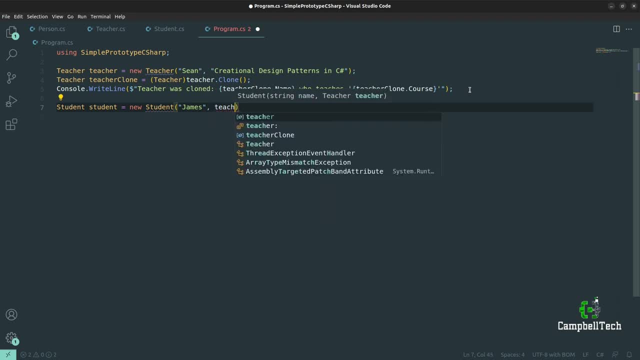 and his teacher is the cloned teacher. now for the class. he'll be done with a and a plugin and a plugin. there we go, hello, hello, hello, and then we're using colonial wellали. we can also create a student clone by invoking going to say, dollar for string interpolation. we can say student was cloned, and then we'll say: 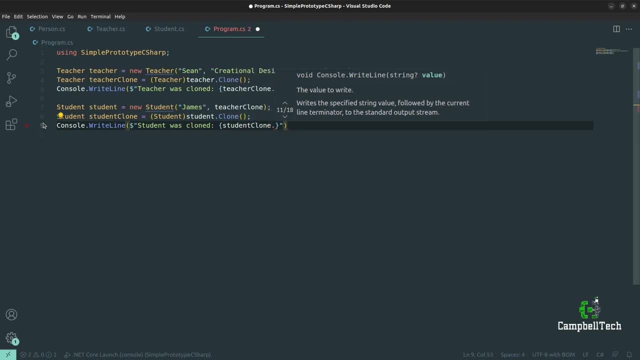 student clone dot name. and then who is enrolled in, let's say, student clone dot, teacher dot name course. i'm not going to print out the course name here again, but you can if you want to. and then we are only cloning both the teacher and student objects. at this moment we're not making any. 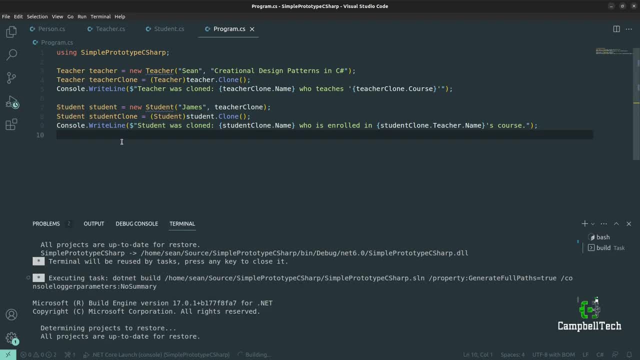 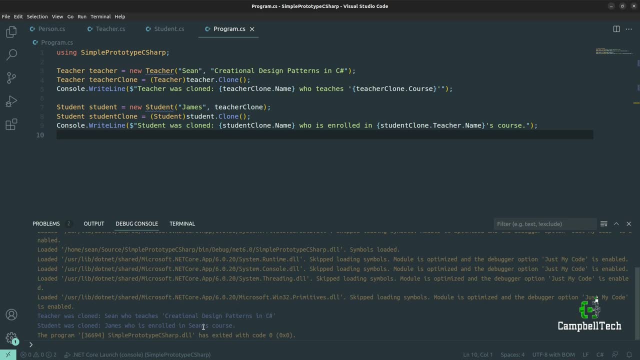 changes yet, so let's just debug now. in the console down here you'll say: teacher was cloned sean, who teaches creation design patterns in c sharp, and student was cloned james, who's enrolled in sean's course. now i don't like to print out to the internal. 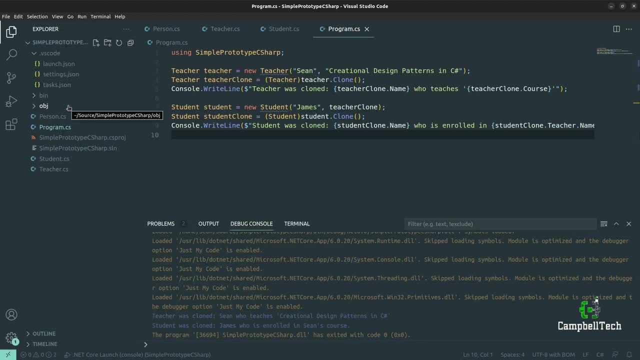 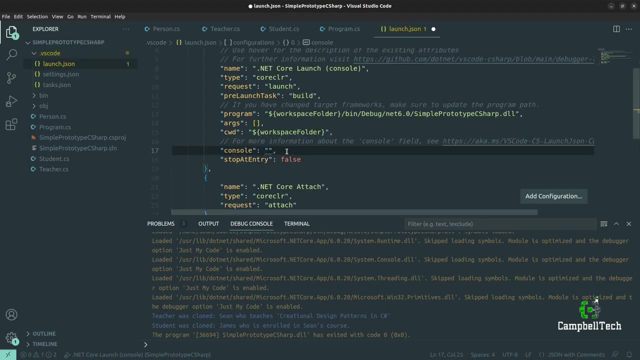 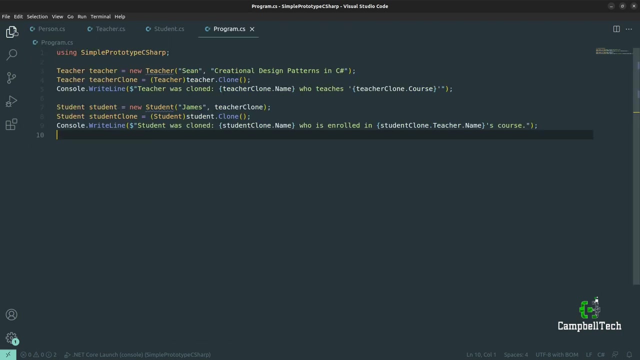 terminal or console like that. so if you want to make it the external terminal, you can go to launchjson and then change internal console to external terminal. okay, so what we can do now is to make a change to the teacher clone. so i'm just going to add a comment here: change the name of the teacher. 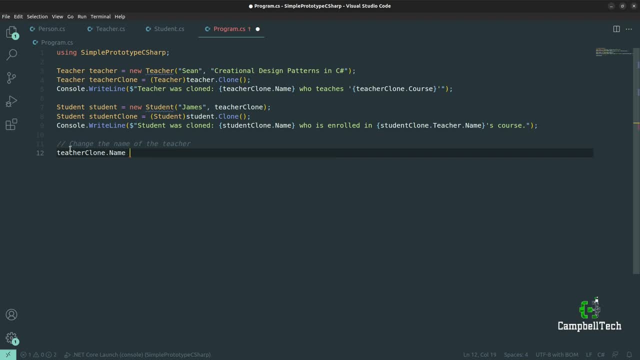 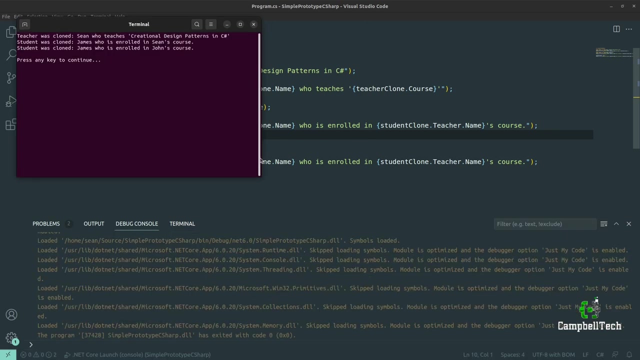 okay. so we'll say: teacher: clone dot name equals. let's change it to john, from sean to john, and then i'm going to print out the student clone part again and you'll see why i'm doing it now. so here it says: teacher was cloned sean, who teaches creation, design patterns and c sharp. 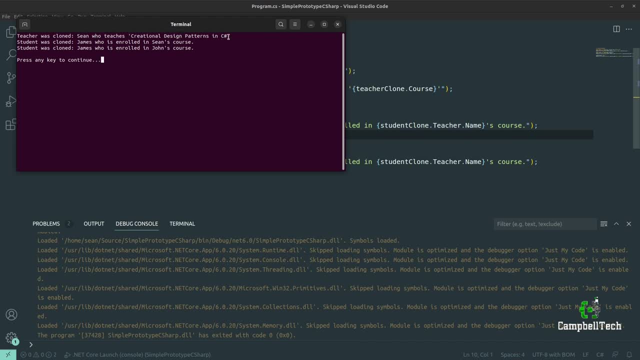 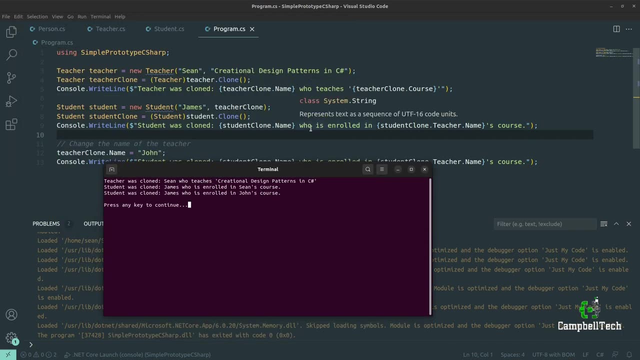 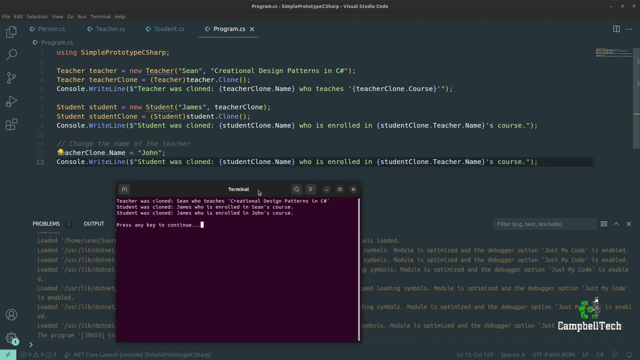 student was cloned: james, who is enrolled in sean's course. that's that second console, that right line, and then the last one there ironically says john's cause. okay, so the reason that this happens is because a shallow copy only complies with a meaningful document script. so it's really going to. 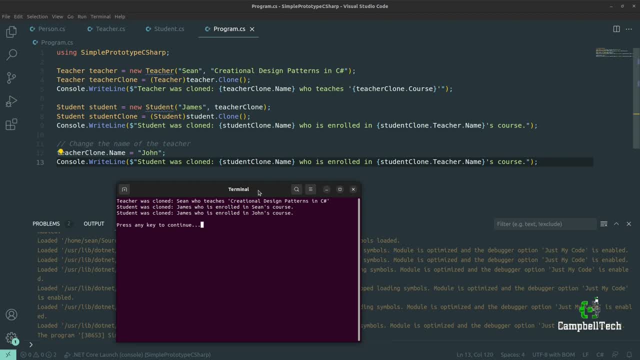 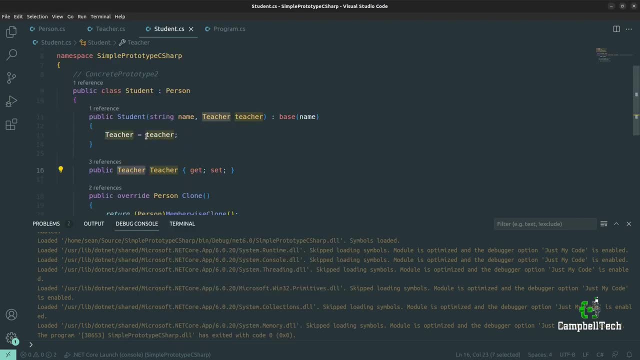 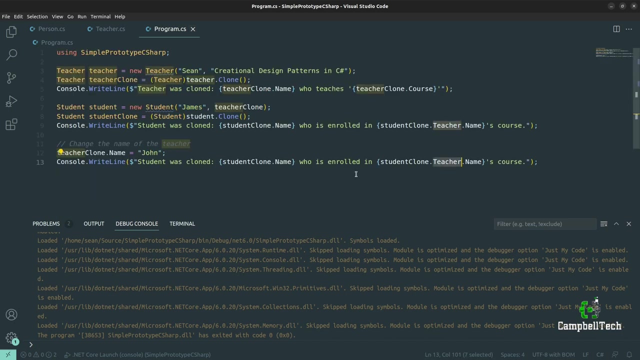 look like a copy. object copies primitive types and not reference types and teacher being a complex object, property on the student object is a reference type and not a primitive type and that's why it's not being cloned or copied. but how do we solve this problem? and the answer is with a deep copy. so 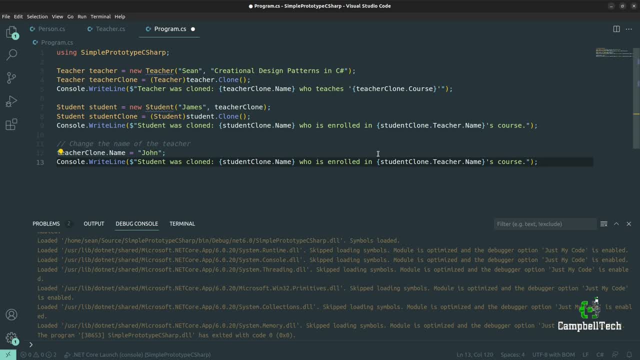 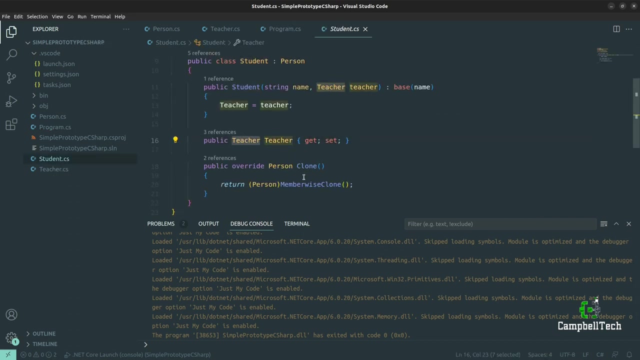 shallow copy, as i mentioned, always only copies the primitive types. but for reference types we need to do a deep copy, and the how part of that is, if we go to our student object, because that is where our reference type is, we can do the following. so, in order for us to make a deep copy, 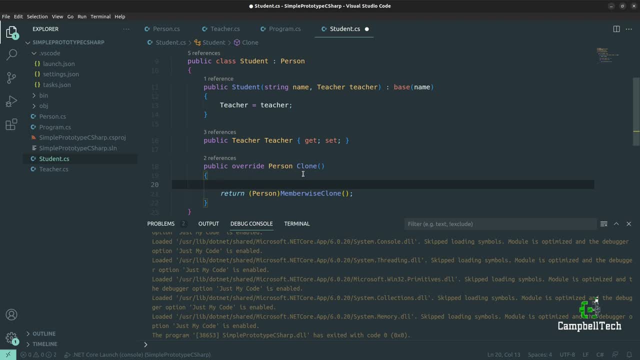 we need to do the following: let's start by creating a student object. so let's say student, call it student clone, and then we'll get it from the member wise clone, but we'll cast it to student this time- member wise clone, okay. and then we can say student clone, dot teacher. this is the important. 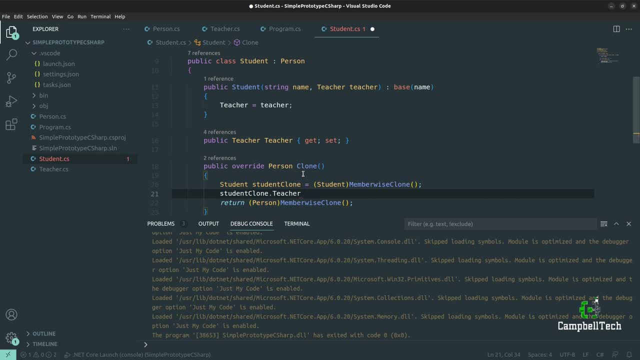 part, because that's the reference type that is not being copied. instead, the reference is being shared across clones. so so we need to specifically and manually create a new teacher object, but we do have this today. so, in order toitt through this, we can change the label code. so i'm going to 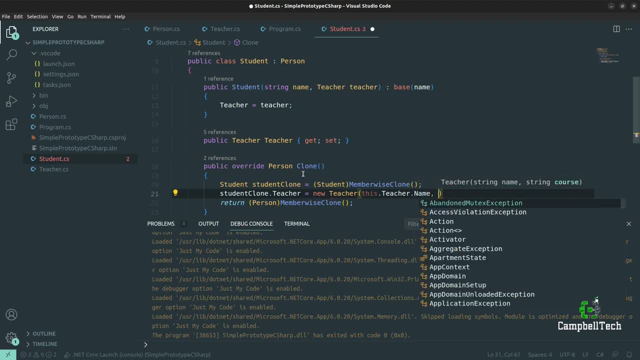 use this calling kids engine Magna namae here and use it to create a new and we have a new student object. now what we're creating is we're actually adding a new copy. so if we go back in our relative, click to to work in and we close our this imprison object. 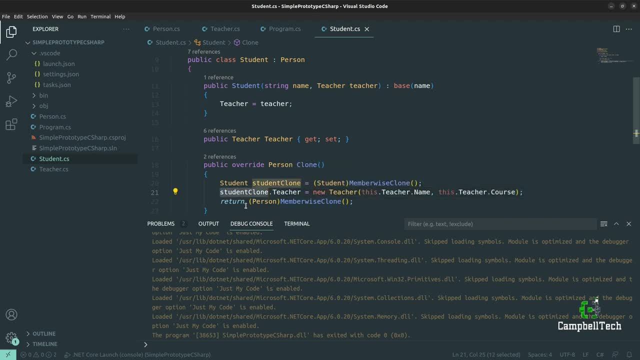 in the user file and you can see that we created this new copy. however, the teacher object isn't seen anymore. you can close this now again with this, Kenneth, that is drawn literally all the other methods that we're returned our user store, going again to using her link to create this style of